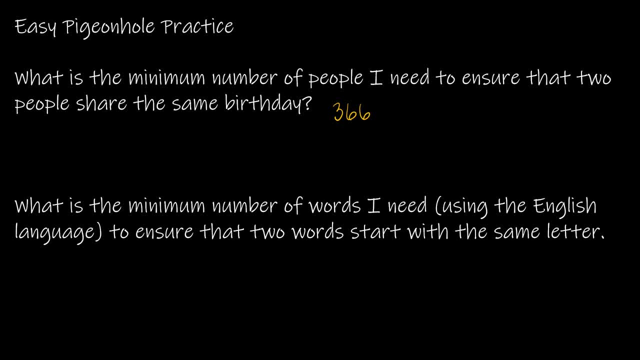 here. Well, I know there are 365 days in a year, but actually there are more days in a year, but actually there are more days in a year, but actually there there's 366 days if you count leap year. February 29th happens once every four years, So there's. 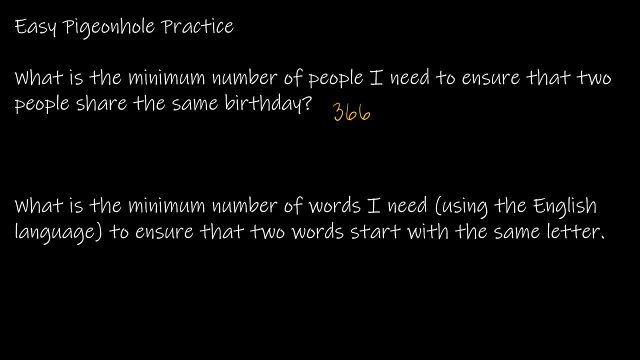 366 different birthdays. So what's the minimum number of people? So if this is K, I need K plus one. So I need 367 people or more. So the minimum number of people would be 367 people. What is the minimum number of words I need, using the English language, to ensure that two words. 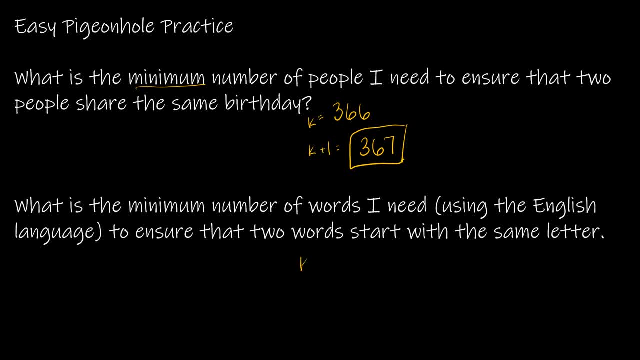 start with the same letter. So again, what's K? How many boxes are there? Well, the boxes in this case are the letters. There are 26 letters of the alphabet in the English language, And K plus one would be that I need 27 or more. Looking now at the generalized pigeonhole principle, 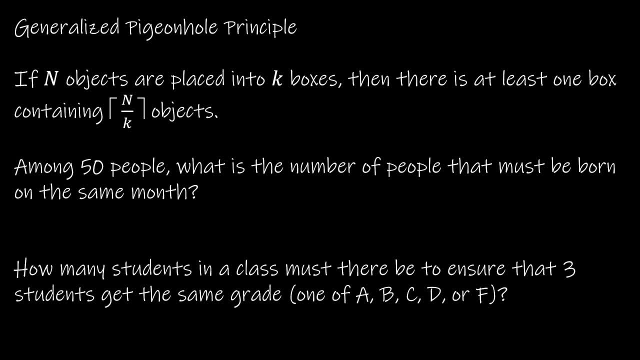 it's really just going to reiterate what we just talked about, but it's going to give us a more mathy way to solve. So here we say: if we have N objects placed into K boxes, then there's at least one box containing 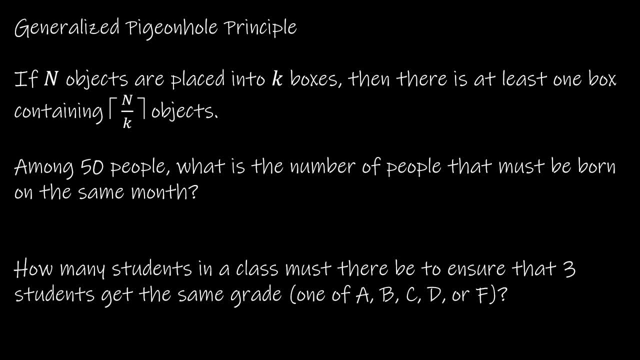 the ceiling function of N divided by K objects. So before we get too far into this, let's just go back to our original example, where I had seven pigeons and I placed them into six boxes. So what the generalized pigeonhole principle says if we have seven objects placed in six boxes. 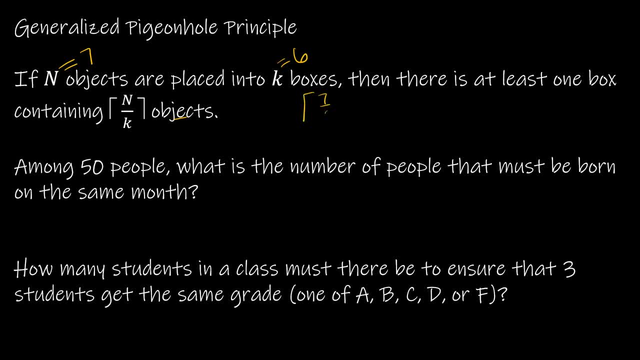 there's at least one box that contains the ceiling function of seven divided by six, which is 1.16.. Ceiling function says what? What is a ceiling function? So just in case we don't understand what a ceiling function is, the ceiling function says: take whatever value you have and round it to. 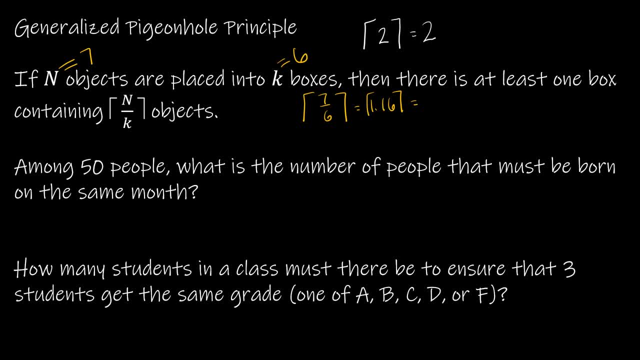 the next integer. Now, 2 already is an integer, and so 2, the ceiling function would be 2.. However, what if I had 2.0001? Almost 2,, but the ceiling function says, okay, that's more than 2,. 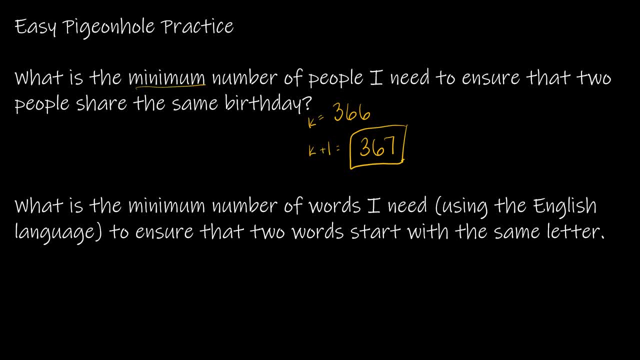 or more, So the minimum number of people would be 367 people. What is the minimum number of words I need, using the English language, To ensure that two words start with the same letter. So again, what's k? How many boxes are there? Well, the boxes in this case are the letters. There are 26. 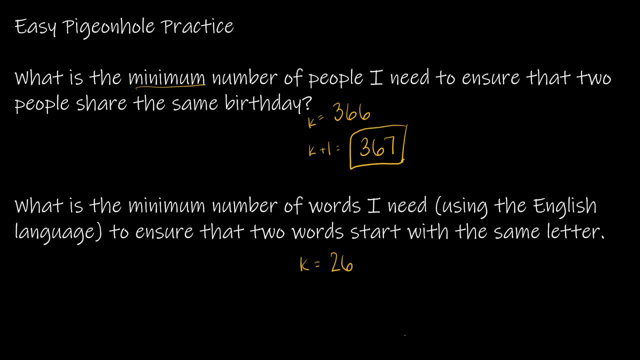 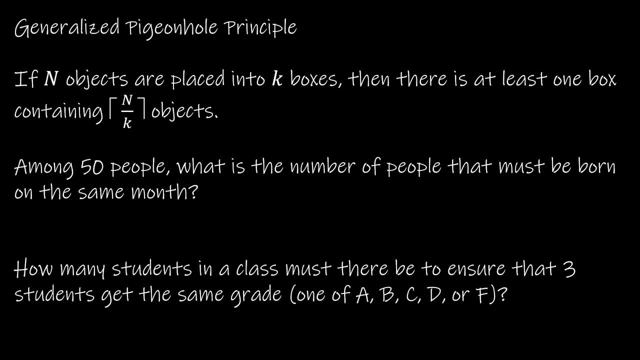 letters of the alphabet in the English language, and k plus one would be that I need 27 or more. Looking now at the generalized pigeonhole principle, it's really just going to reiterate what we just talked about, but it's going to give. 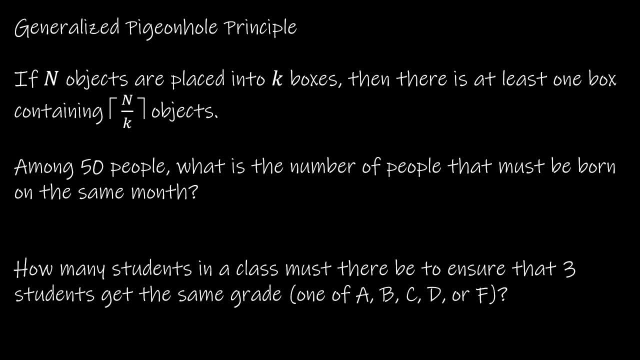 us a more mathy way to solve. So here we say: if we have n objects placed into k boxes, then there's at least one box containing the ceiling function of n divided by k objects. So before we get too far into this, let's just go back to our original. 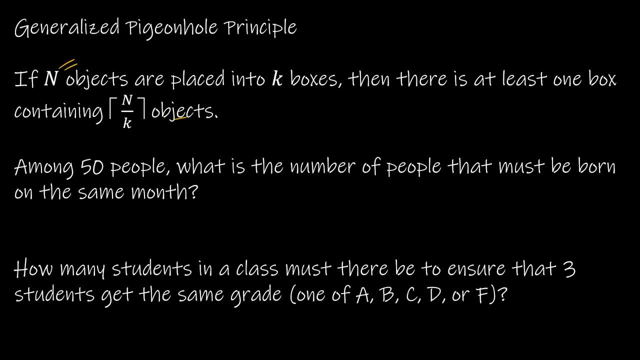 example, where I had seven pigeons and I placed them into six boxes. So what the generalized pigeonhole principle says is that the number of pigeons in the objects that we have placed into the box is at least one. This 2 already is an integer, and so 2, the ceiling function would be 2.. However, what if I had? 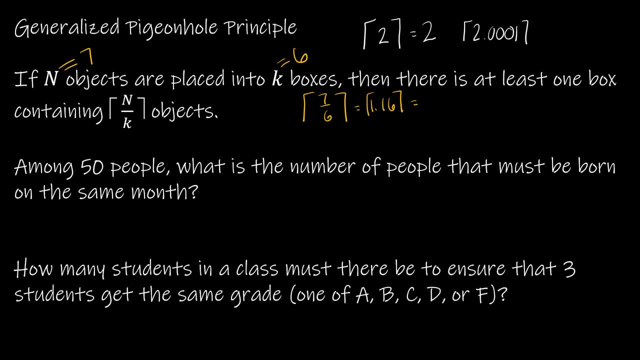 2.0001? Almost 2, but the ceiling function says okay, that's more than 2, so now you have to round up to the next integer. Same thing if I had 2.99, that is less than 3,. so when I round it up, 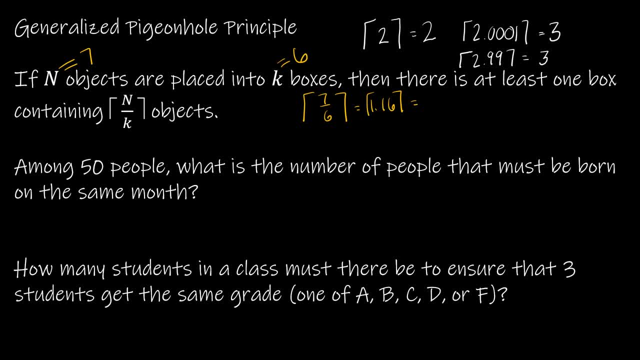 to the next integer, it's going to be 3.. So back to our example. what does our pigeonhole principle tell us? It says there's going to be at least one box with two objects. Well, that's what we had said before. We said, hey, if we have seven pigeons, we have six pigeonholes. then there's at least. 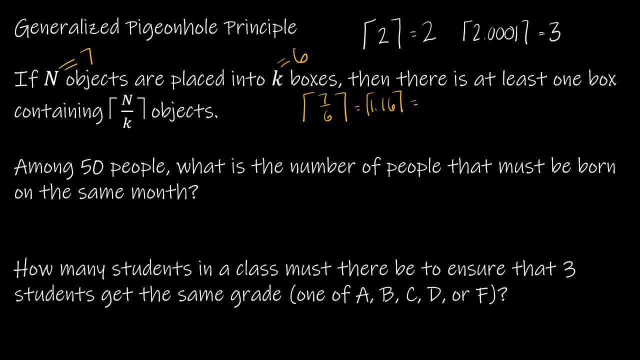 so now you have to round up to the next integer. Same thing. if I had 2.99, that is less than 3, so when I round it up to the next integer, it's going to be 3.. So back to our example. what does our pigeonhole principle tell us? It says there's going to be at. 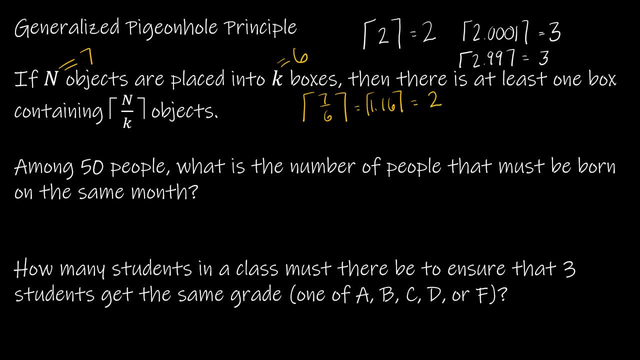 least one box with two objects. Well, that's what we had said before. We said, hey, if we have seven pigeons, we have six pigeonholes. then there's at least one pigeonhole that has two pigeons in it, and that's exactly what this is saying. Let's take a look at a 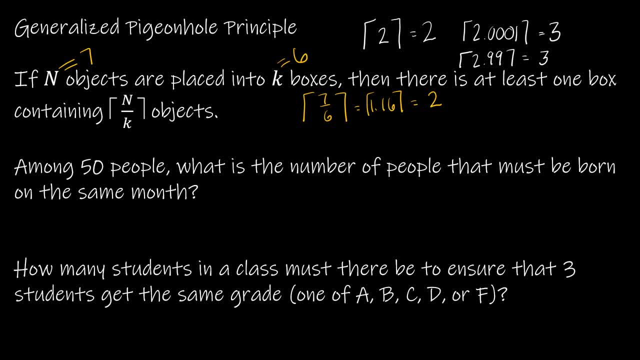 very straightforward example, straightforward application: If we have 50 people, what's the number of people that must be born on the same month? So again, 50 people would be 50 objects, that's n, and the number of people that must be born on the same month, that's the number of boxes. 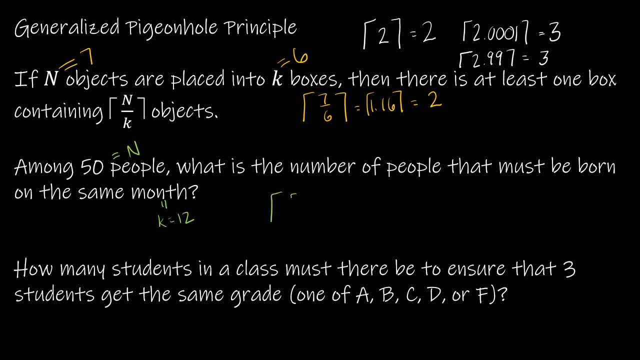 so k is 12.. So really we're just saying: let's take 50 divided by 12,, which gives us 4.16, regardless of the number of boxes. So let's take 50 divided by 12,, which gives us 4.16,. 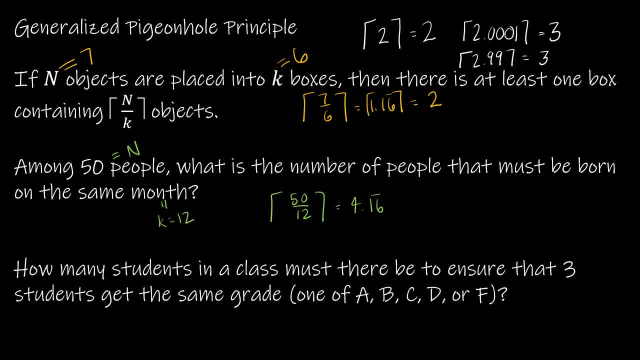 and that was also repeating up there- and using the ceiling function, we round that to five. So if we have 50 people, then the number of people that must be born on the same month is five. Now, it could be more than that, but we're saying worst case scenario, five. Now the next. 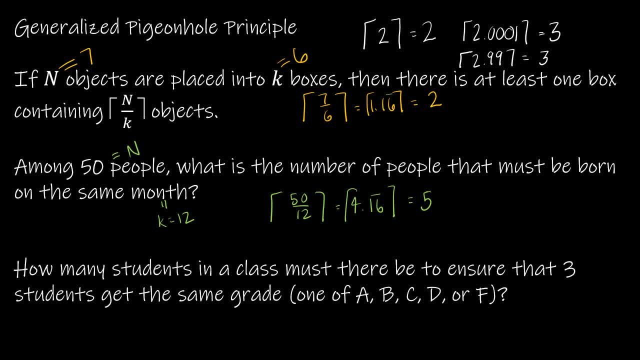 question a little bit trickier still. the same pigeonhole principle, but a little bit more complicated. So here we have a pigeonhole principle and we're saying: let's take 50 people that must be born on the same month. So here we have the number of students in a class must. 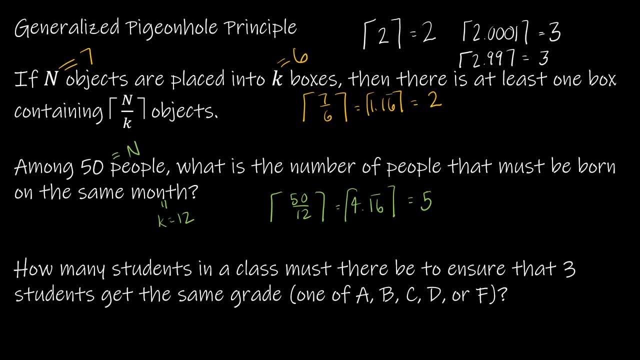 there be to ensure that three students get the same grade of A, B, C, D or F. So hopefully we can see that this would be the boxes We're trying to put people into the boxes of which grade they get. This is going to be the outcome. So if I were to set this up, it would look more. 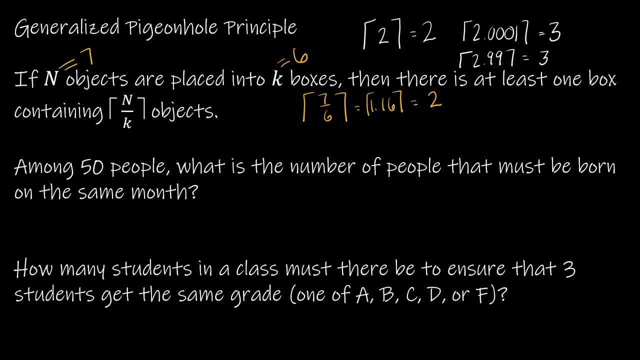 one pigeonhole that has two pigeons in it, and that's exactly what this is saying. Let's take a look at a very straightforward example, straightforward application: If we have 15 pigeons, we have 6 pigeons in it, and we have 6 pigeons in it, and we have 6 pigeons in it and 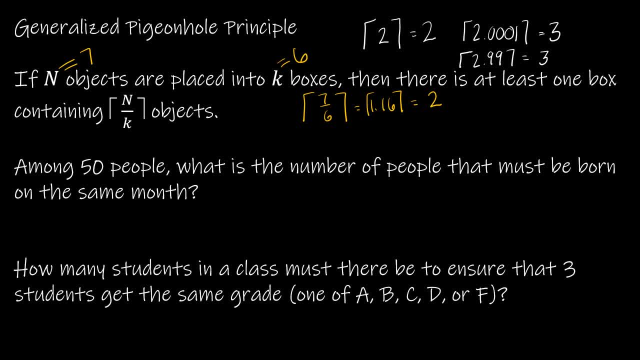 what's the number of people that must be born on the same month. So again, 50 people would be 50 objects, that's n, and the number of people that must be born on the same month, that's the number of boxes. so k is 12.. So really we're just saying: let's take 50 divided by 12, which gives 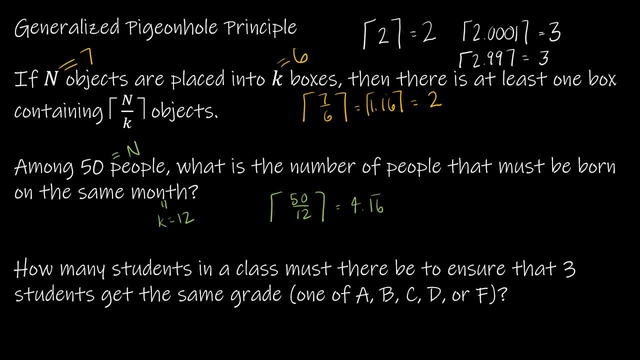 us 4.16. repeating- and that was also repeating up there- And using the ceiling function, we round that to 5.. So if we have 50 people, then the number of people that must be born on the same month is 5.. Now, it could be more than that, but we're saying worst. 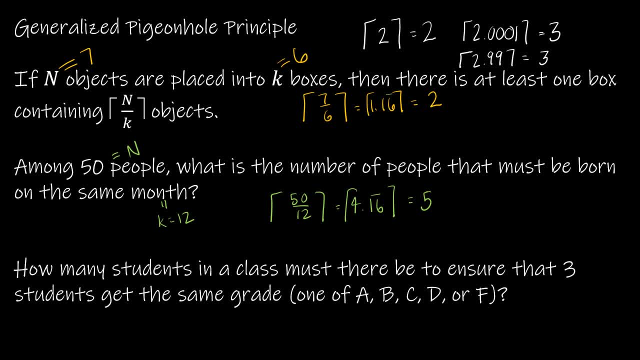 case scenario 5.. Now the next question, a little bit trickier. still the same pigeonhole principle, but a little bit more complicated. So here we have the number of students in a class. must there be to ensure that three students get the same number of students in a class? 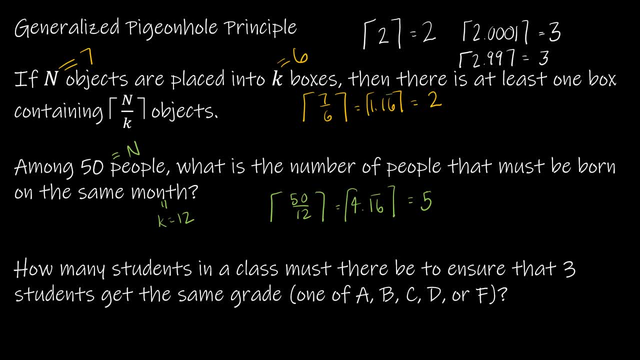 The same grade of A, B, C, D or F. So hopefully we can see that this would be the boxes We're trying to put people into, the boxes of which grade they get. This is going to be the outcome. So if I were to set this up, it would look more like: 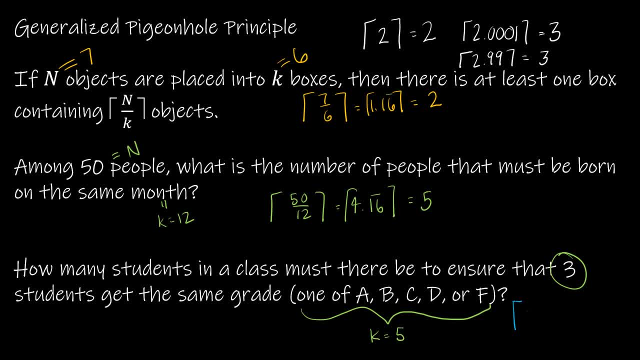 oops, that's a bad ceiling. n divided by 5 is equal to 3.. Now, this is a good thing. This is a good thing, But it's not as straightforward to solve this, because if I were solving this, this would say: 5 times 3 is 15.. But that's not what I want. 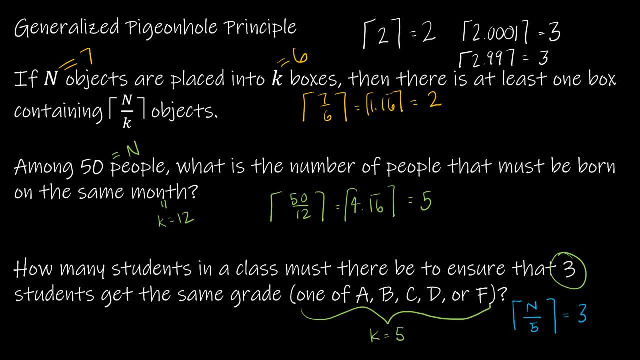 because this is a ceiling function. So before we talk about the mathematical way to solve this, let's just work it out just by reasoning. I'm going to erase this If I were to have again. we're looking for ensure that there are three that get the same grade. Let's look at worst case scenario. 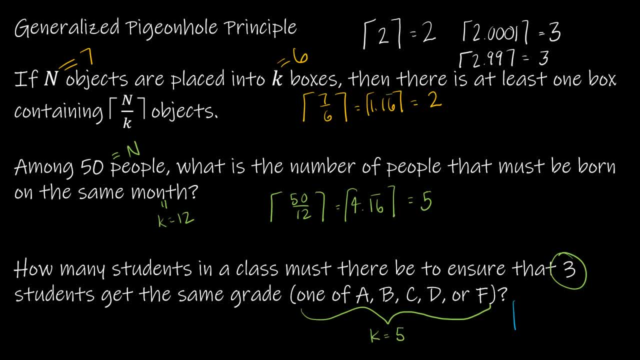 like: oops, that's a bad ceiling. n divided by five is equal to three. Now it's not as straightforward to solve this, because if I were solving this, this would say: five times three is 15, but that's not what I want, right. 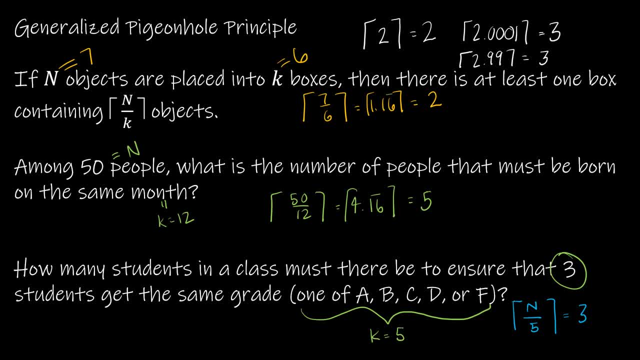 Because this is a ceiling function. So before we talk about the mathematical way to solve this, let's just work it out just by reasoning. If I have, I'm going to erase this If I were to have again. we're looking for ensure that there are three that get the same grade. Let's look at worst. 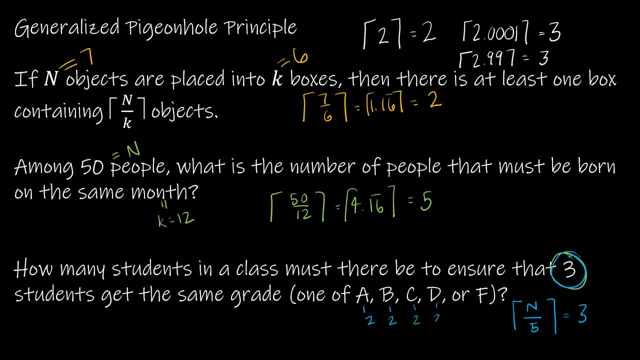 case scenario is: everybody, or every box has two students. So I have two students with an A, two with a B, two with a C, two with a D, two with an F, That's 10 students. Can I ensure? 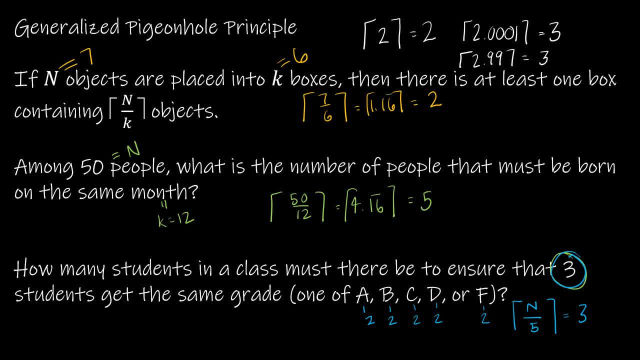 then, that there are three students that get the same grade with 10?? No, but by the pigeonhole principle, if I add one more to that which is 11, now I can ensure that three students get the same grade because that last pigeon or that last student needs to go in one of the boxes that 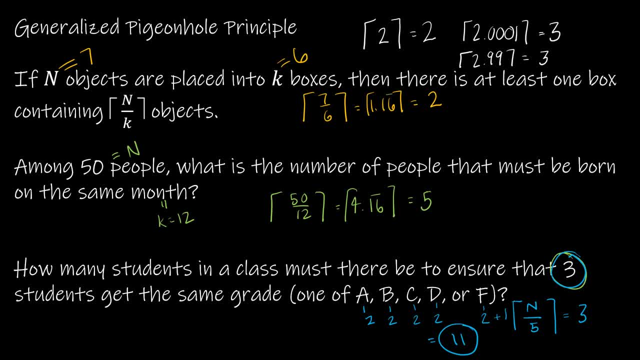 already has two people in it, So 11 is the correct answer. So now the question becomes: how do I solve that mathematically? Well, because we're dealing with the ceiling function. what I want to do is say that I want one less than this. So I'm going to look at what happens. 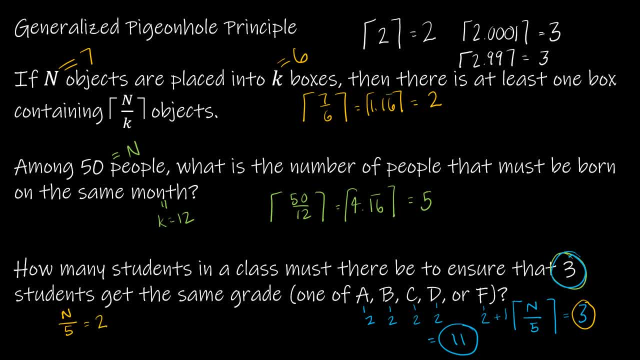 if I take n divided by 5 equals 2.. Well, obviously, if I multiply each side by 5, I get n is equal to 10.. Now, is that the answer? No, because we already talked about the fact that. 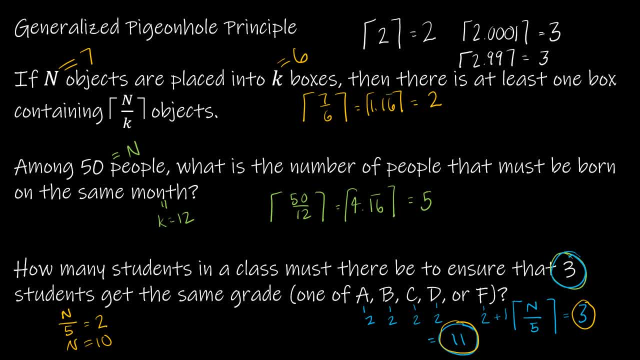 the answer is 11.. So how can I set this up mathematically? I can say n minus 1.. So really, I'm taking one away from here and one away from here. And now, if I solve this, let's say if I- 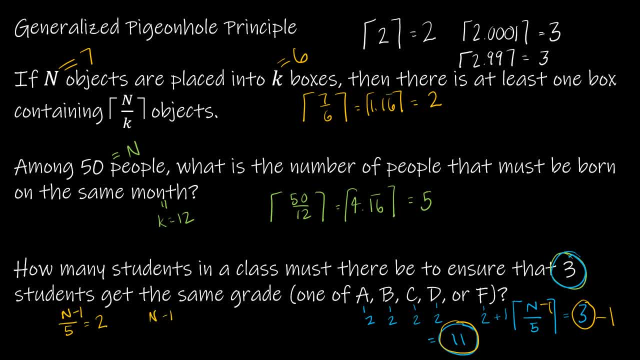 multiply each side by 10, I get n minus 1.. So I'm taking one away from here and one away from here. Or by 5, I get n minus 1 is equal to 10.. I add one to each side, I get that I must have 11.. So 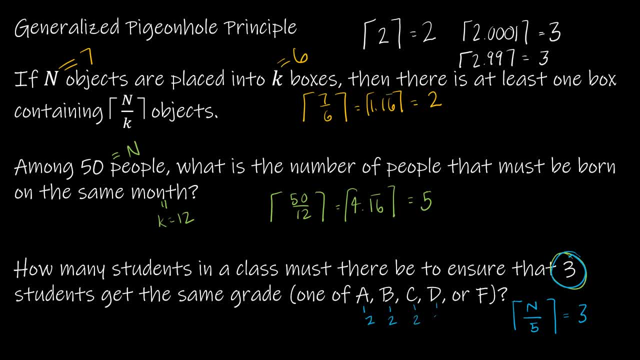 Let's look at worst case scenario. Let's look at worst case scenario. Let's look at worst case scenario. scenario is: everybody, or every box, has two students. So I have two students with an A, two with a B, two with a C, two with a D, two with an F. That's 10 students. Can I ensure then? 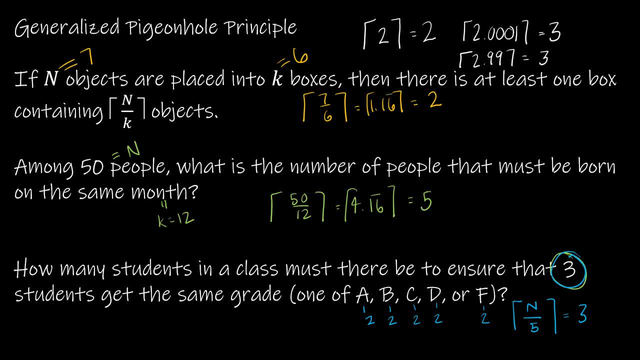 that there are three students that get the same grade with 10?? No, but by the pigeonhole principle, if I add one more to that, which is 11, now I can ensure that three students get the same grade because that last pigeon or that last student needs to go in one of the boxes that already has. 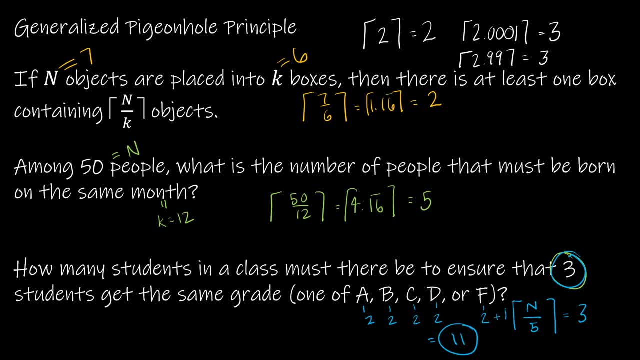 two people in it, So 11 is the correct answer. So now the question becomes: how do I solve that mathematically? Well, because we're dealing with the ceiling function. what I want to do is say that I want one less than this. So I'm going to look at what happens. if I take n divided by 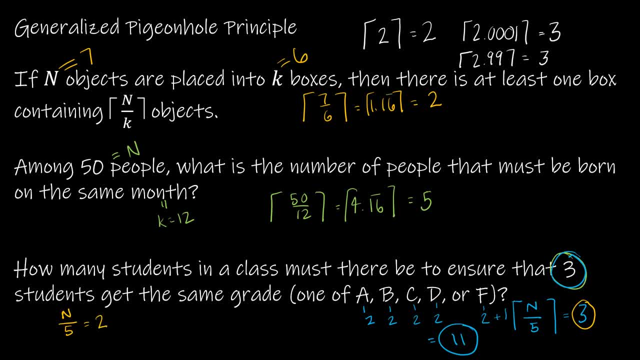 5 equals 2.. Well, obviously, if I multiply each side by 5, I get n is equal to 10.. Now, is that the answer? No, because we already talked about the fact that the answer is 11.. 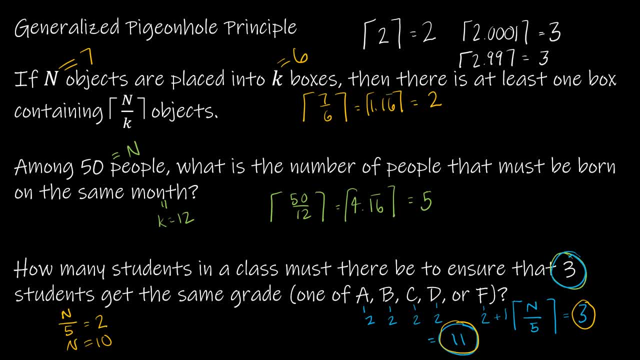 So how can I set this up mathematically? I can say n minus 1.. So really, I'm taking one away from here and one away from here. And now, if I solve this, let's say if I multiply each side by: 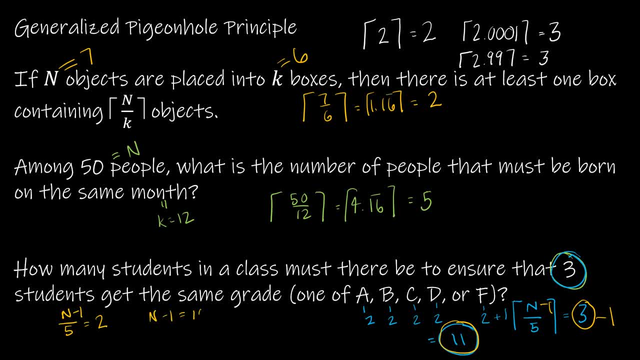 10 or by 5,, I get n minus 1.. So I can say n minus 1.. So I can say n minus 1.. So I can say n minus 1.. n minus 1 is equal to 10.. I add one to each side, I get that I must have 11.. So that's one way to do. 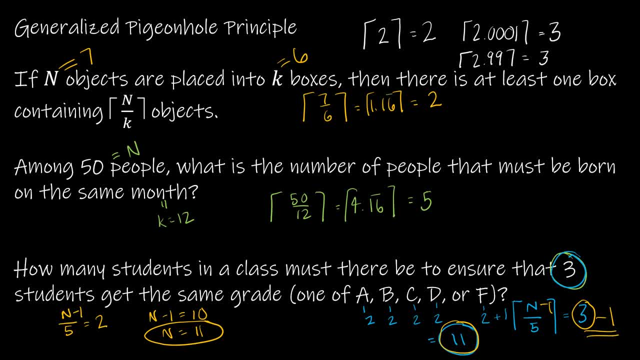 it Again, because we're dealing with the ceiling function. I can take one away from here and one away from here, And really the one away from the end is so that at the end I can add one more, just like I did here. Let's take a look at another practice, And this is a two-part question. 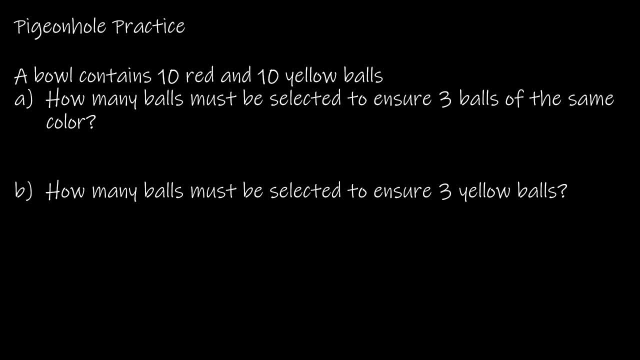 This one. I have a bowl that contains 10 red and 10 yellow balls, And I want to know how many balls must be selected to ensure three balls of the same color. So hopefully we can see that this is almost exactly the same type of question that we just 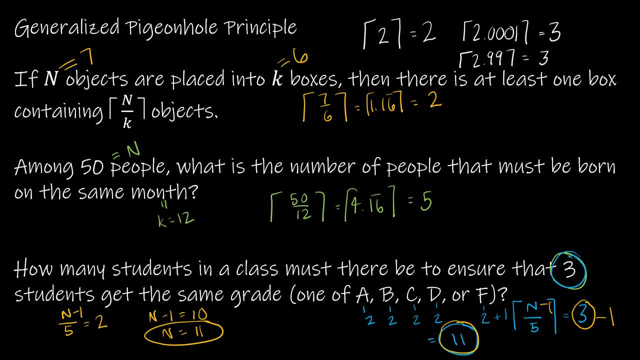 that's one way to do it. Again, because we're dealing with the ceiling function, I can take one away from here and one away from here, And really the one away from the end is so that at the end I can add one more, just like I did here. Let's take a look at another practice. 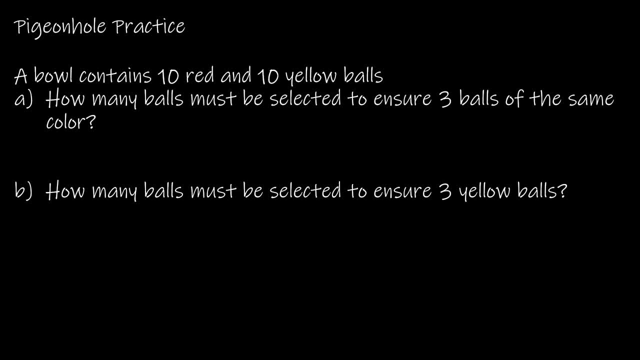 and this is a two-part question, This one: I have a bowl that contains 10 red and 10 yellow balls, And I want to know how many balls must be selected to ensure three balls of the same color. So hopefully we can see that this is almost exactly the same type of question that we just 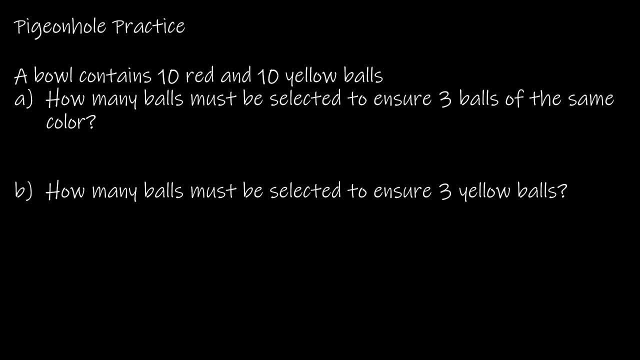 did So I can look at worst-case scenario and say, okay, if the first one was red, and then the second one was red, and then the next one was yellow, and the next one was yellow, now I'm in a position where the next one is going to have to make it. 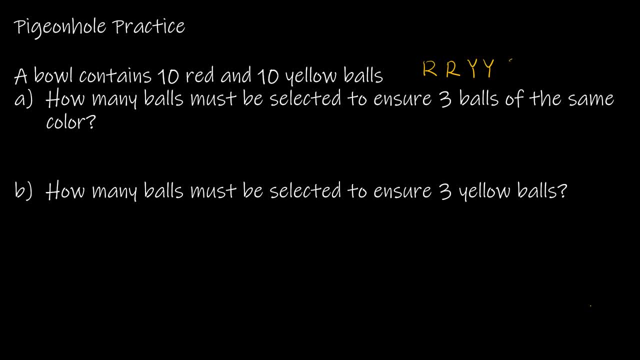 so that I have three red or three yellow. So the correct answer is five. Now, obviously I don't want to have to reason through it like that, I want to just be able to do the math. So again we're saying we have two bins and we're solving for n and we want to be 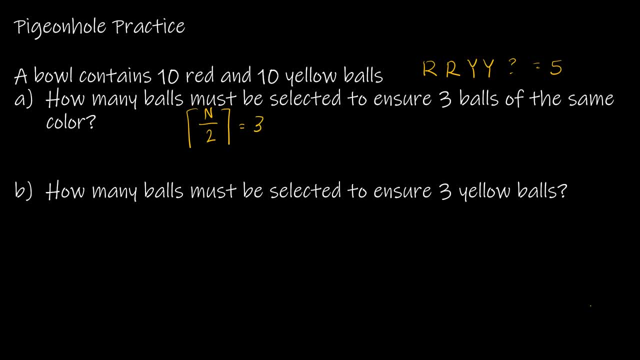 three balls of the same color. So how did we do this? before We said, let's say, n minus one, divided by two, was equal to three minus one. So we took one away from n and one away from the result, since we're dealing with the ceiling function. 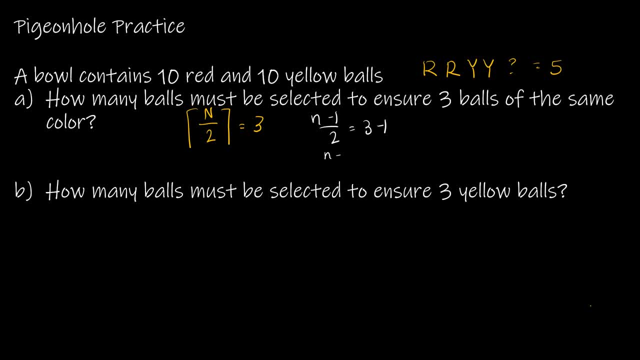 So we get n minus one over two is equal to two. Multiplying each side by two, I get n minus one equals four. Adding one, I get n is five. And again, I showed a lot of work there, but you get. 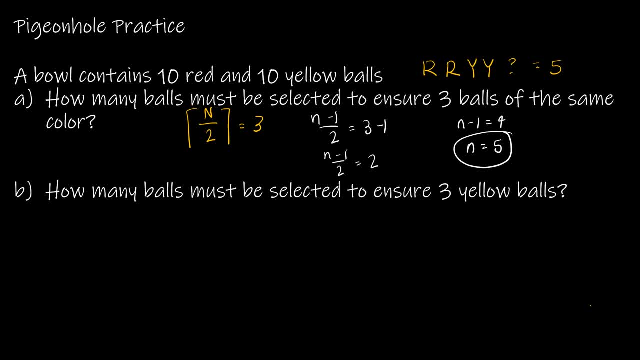 the idea that that's a really easy way to go about solving a question like that. Now the next one can't really be solved. So let's say that we have two bins and we're solving for n minus one with the pigeonhole principle in a direct application. So it's saying how many balls? 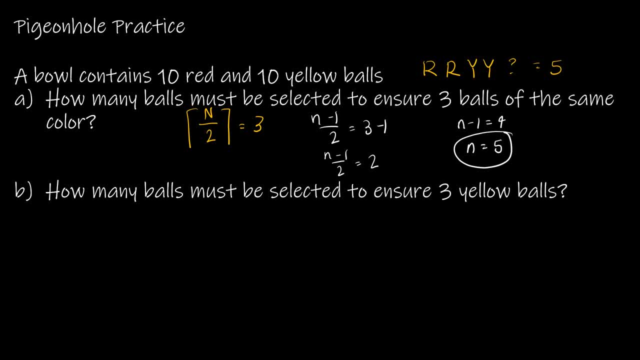 must be selected to ensure three yellow balls. So again I'm going to be thinking about worst case scenario. Worst case scenario says I'm going to pick a red and then a red, and then a red, and then a red, all the way through until I run out of reds. Now we could talk probability. 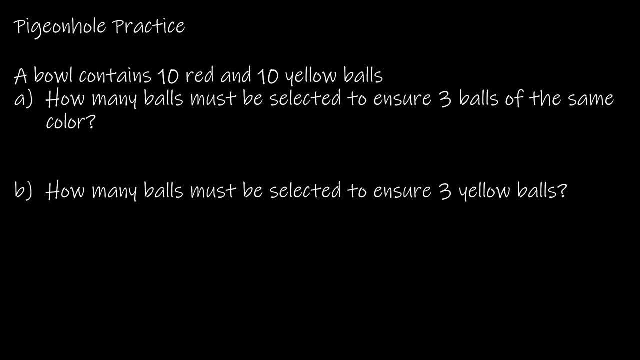 did So I can look at worst-case scenario and say, OK, if the first one was red, and then the second one was red, and then the next one was yellow, and the next one was yellow. now I'm at a position. 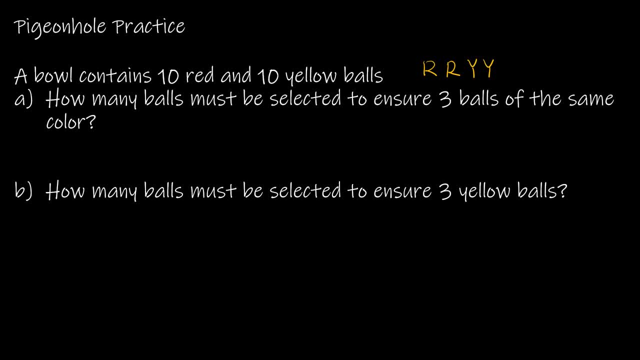 where the next one is going to have to make it so that I have three red or three yellow balls, So the correct answer is five. Now, obviously, I don't want to have to reason through it like that, I want to just be able to do the math. So again we're saying we have two bins. 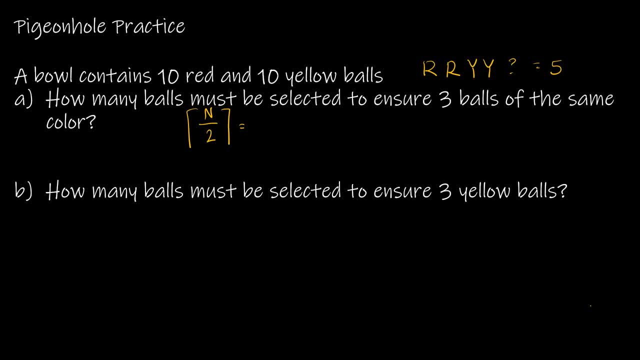 and we're solving for n and we want to be three balls of the same color. So how did we do this? before We said, let's say, n minus 1 divided by 2 was equal to 3 minus 1.. So we took one away from n. 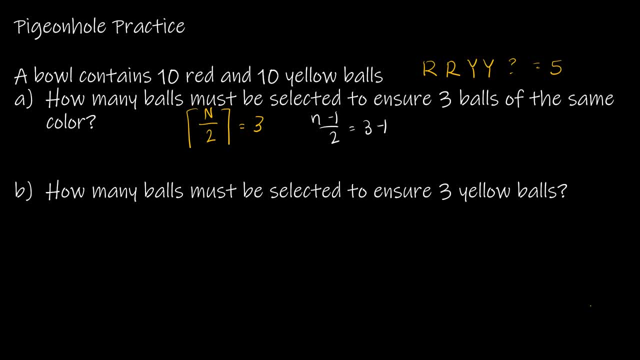 and one away from the resultant, And we're going to do that again. So we're going to do that again, since we're dealing with the ceiling function. So we get n minus 1 over 2 is equal to 2.. Multiplying each side by 2, I get n minus 1 equals 4.. Adding 1, I get n is 5.. And again. 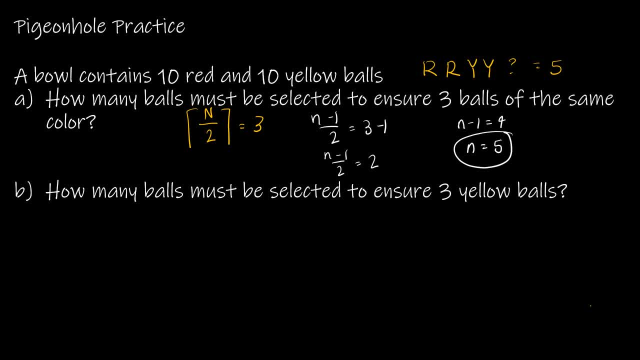 I showed a lot of work there, but you get the idea that that's a really easy way to go about solving a question like that. Now, the next one can't really be solved with the pigeonhole principle in a direct application. So it's saying how many balls must be selected to ensure. 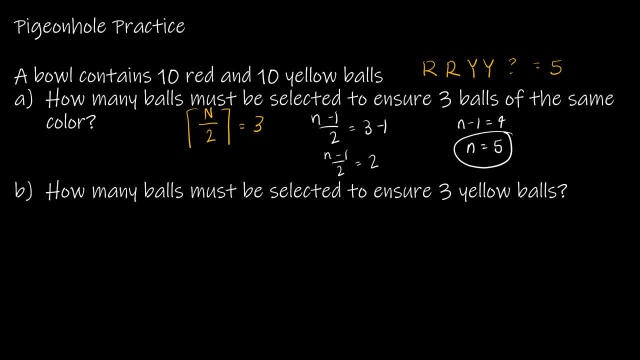 three yellow balls. So again I'm going to be thinking about worst case scenario. Worst case scenario says I'm going to pick a red, and then a red, and then a red, and then a red, all the way through until I run out of reds. Now we could talk probability, but that's not very. 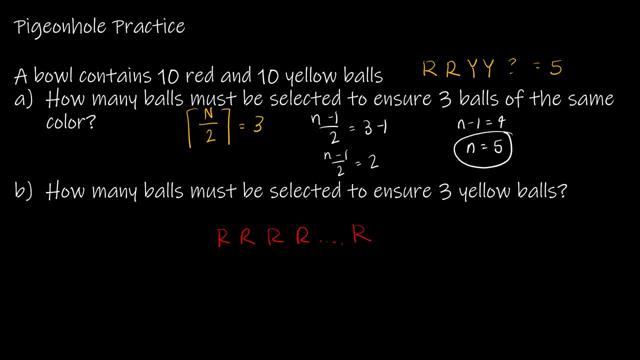 probable but possible. So basically, I could have all 10 reds before I draw a yellow and then I'm going to get a yellow and a yellow and a yellow. So the correct answer is 13. And there's really no mathematical way for you to apply. 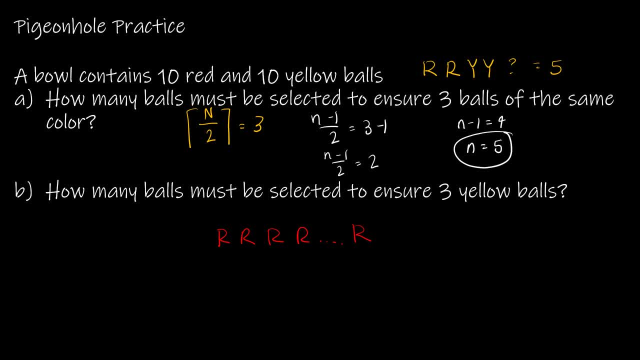 that's not very probable but possible. So basically, I could have all 10 reds before I draw a yellow and then I'm going to get a yellow and a yellow and a yellow. So the correct answer is 13. And there's really no mathematical way for you to apply. 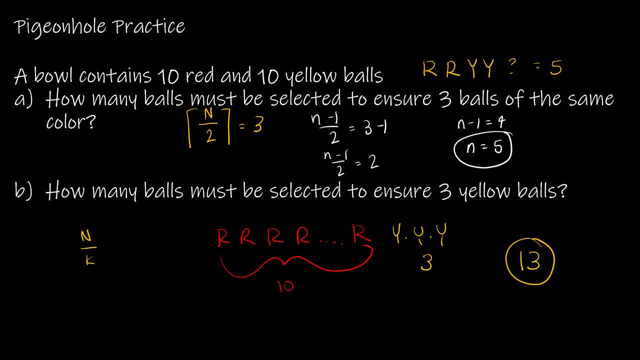 n divided by k- what we just talked about with pigeonhole principle. There's really no way to do that except to say you're going to draw all the reds first and then you're going to start adding reds. So that's really not a mathematical way for you to apply. n divided by k. 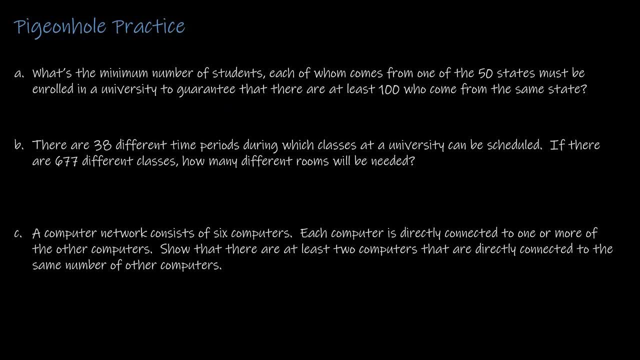 Here are three questions I would like you to try on your own, which are just different applications of the pigeonhole principle. When you are ready, press play to see how you did For the first one. this is structured in the same way that we have done a couple of other questions. 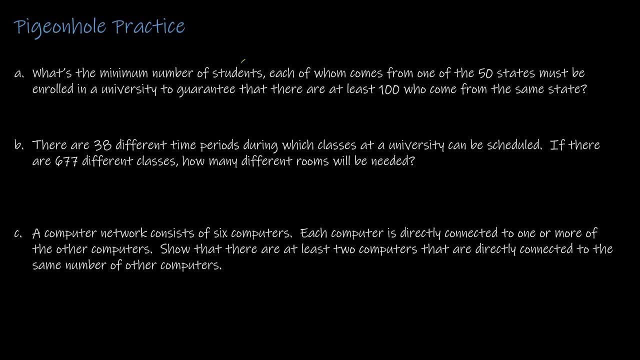 We are solving for n. We're saying: what's the minimum number of students n, each of whom comes from one of the 50 states? that would be considered the number of bins that we have, or boxes enrolled in a university, to guarantee at least 100.. So if I were to set this up, I would say: 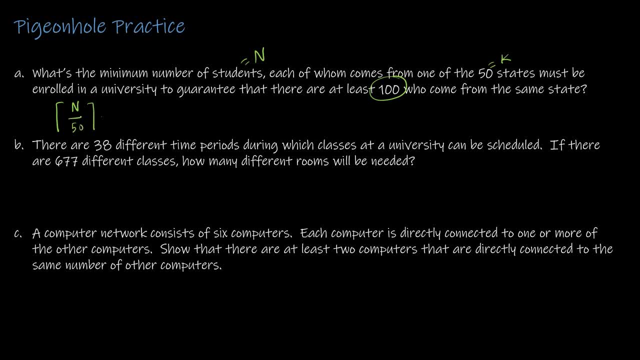 n divided by 50 equals 100.. And then remember: the easiest way to solve this is to say: n minus 1, divided by 50, is equal to 100 minus 1, which is 99.. To solve, I would multiply each side by 50. 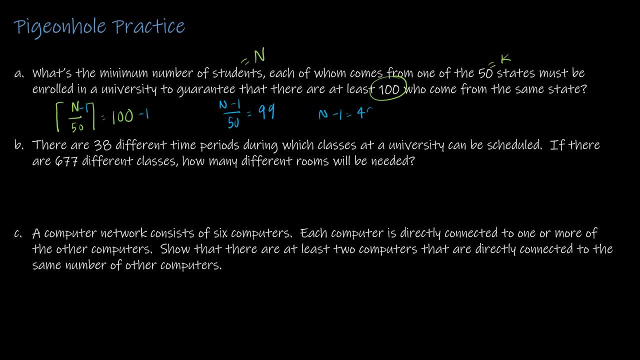 So I would get: n minus 1 is equal to 4,950, so I would need adding one to each side n to be 4,951.. So the question is: I would need a minimum of 4,951 students to ensure that I have at least 100 from the same state. 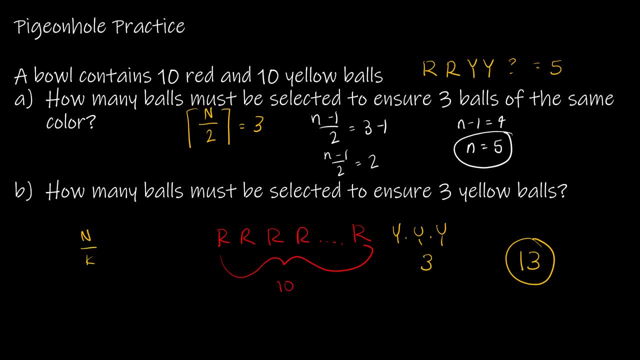 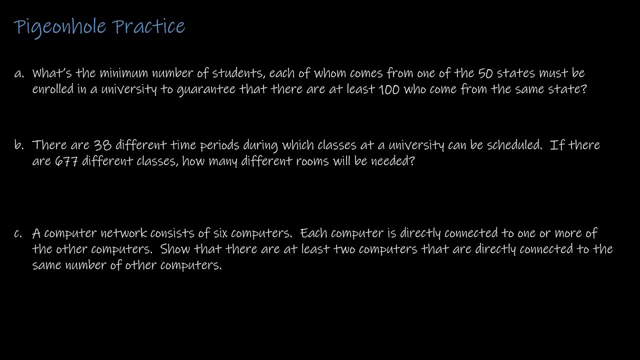 n divided by k- what we just talked about with pigeonhole principle. There's really no way to do that except to say you're going to draw all the reds first and then you're going to start adding yellow balls. Here are three questions I would like you to try on your own, which are just different. 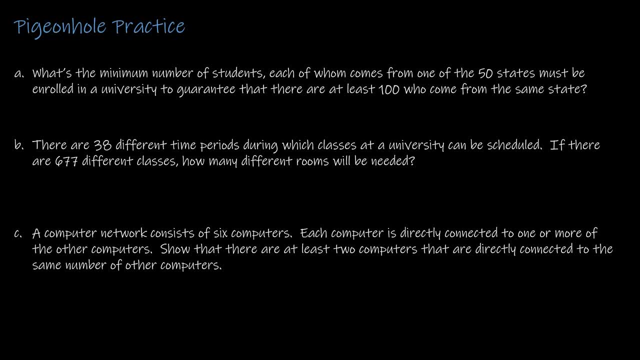 applications of the pigeonhole principle. When you are ready, press play to see how you did For the first one. this is structured in the same way that we have done a couple of other questions We are solving for n. We're saying what's the minimum number of students n, each of whom comes? 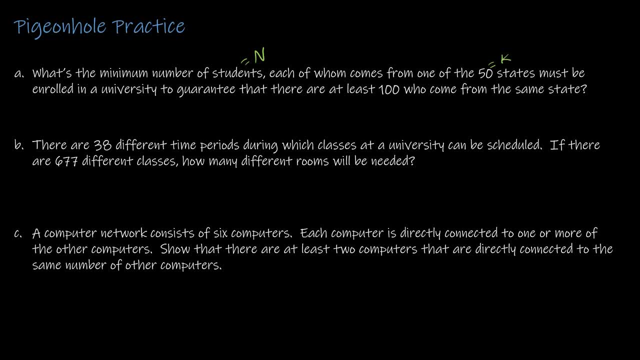 from one of the 50 states, That would be considered the number of bins that we have or boxes Enrolled in a university to guarantee at least 100.. So if I were to set this up, I would say n divided by 50 equals 100. And then remember, the easiest way to solve this is to say: 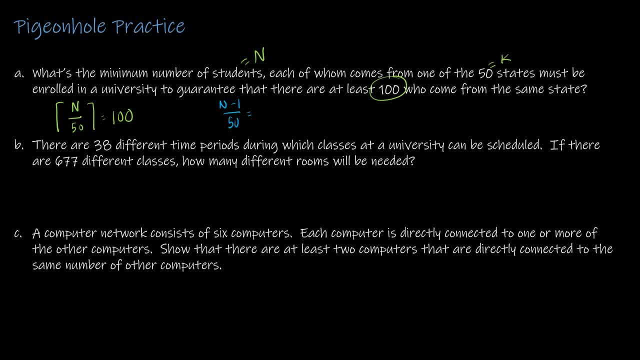 n minus 1, divided by 50, is equal to 100 minus 1, which is 99.. To solve, I would multiply each side by 50.. So I would get n minus 1.. is equal to 4,950, so I would need adding one to each side, n, to be 4,951.. So the question is: 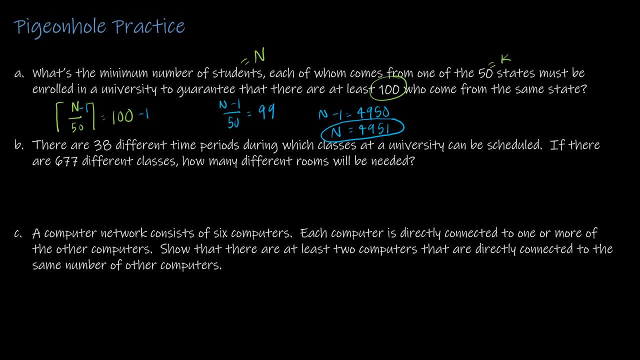 I would need a minimum of 4,951 students to ensure that I have at least 100 from the same state. For b, there are 38 different time periods during which classes at a university can be scheduled. If there are 677 different classes, how many different rooms will be needed? 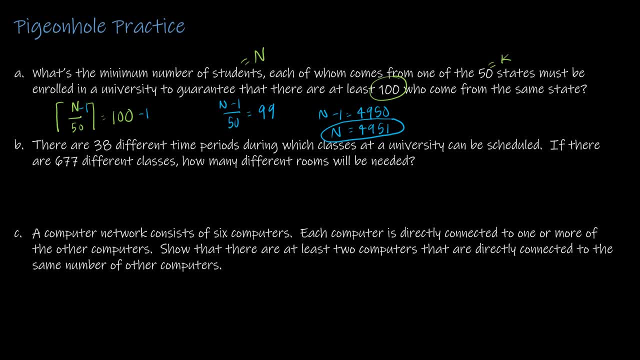 So we have 38 different time periods and 677 classes. This is a straight up application, so I'm going to take 677 divided by 38, which gives me 17.8157. blah, blah, blah. Doesn't matter, I know that that rounds up to 18.. So I will need 18 different rooms in order to make that.